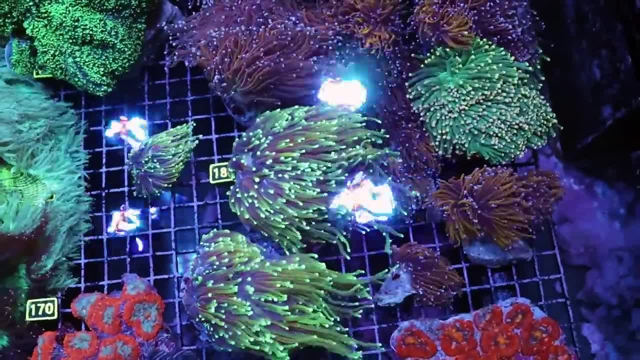 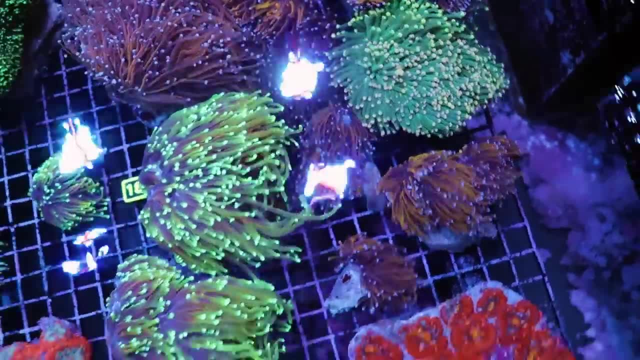 Torch coral pulls right back into its skeleton And they don't look very good. Hold on, I think I have a dying one here, Because I always show you guys That's the next annually purchase. I need to use the good and the bad. Yep, I knew I had one over here. This is not good. 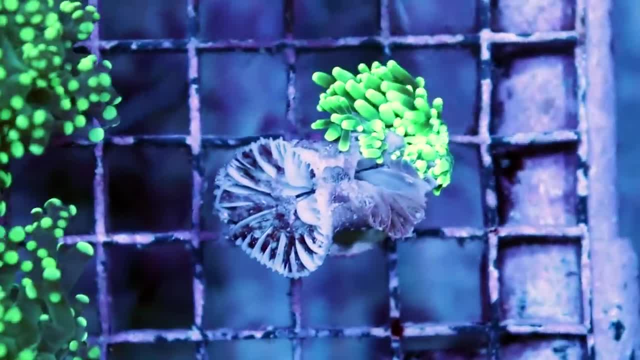 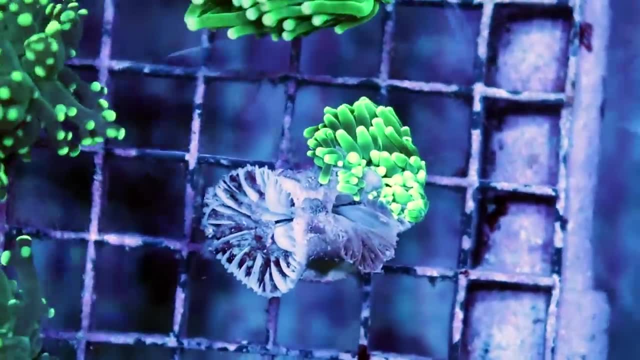 Don't ever buy a torch coral over here that looks like this. People call it brown jelly. There's no brown jelly. I'll do another video on that. I don't like rocking the boat too much. I have some controversial opinions on stuff Like brown jelly, I think, is one of them. 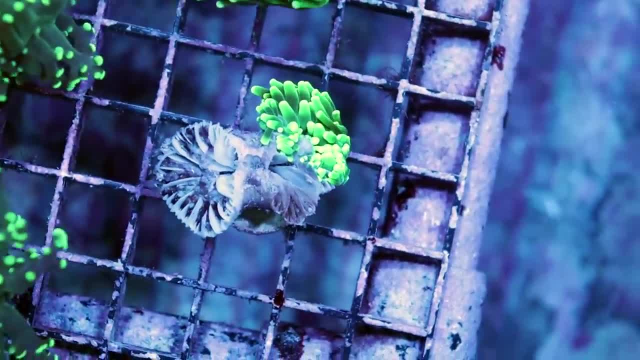 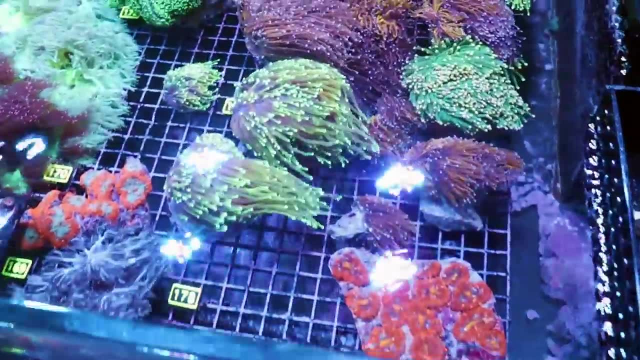 I think people confuse dying torch coral for brown jelly. That's just your torch coral dying. I'll do a whole other video on my thoughts on brown jelly But not to get sidetracked, the one looks like these are what very, very healthy ones look like. I was afraid. 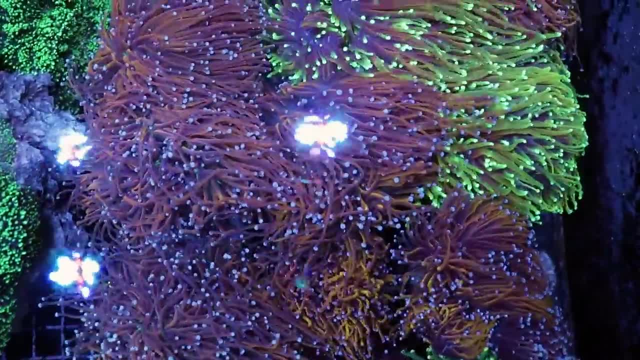 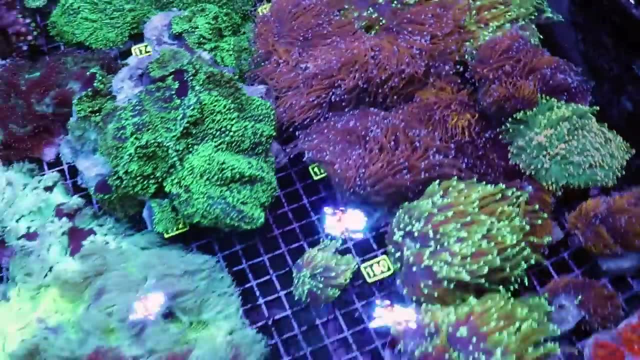 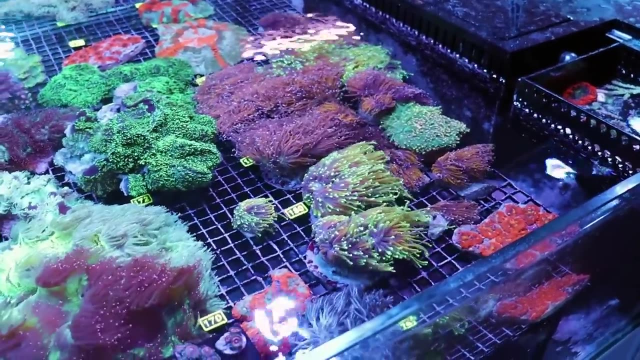 we were gonna lose some, so I wanted them to hang out and chill and open up and just get looking fantastic before I picked up the camera to share with you them the probably- I'm gonna say probably- the nicest assortment of torch corals we've gotten in a long time, maybe ever. it's hard to remember because we're 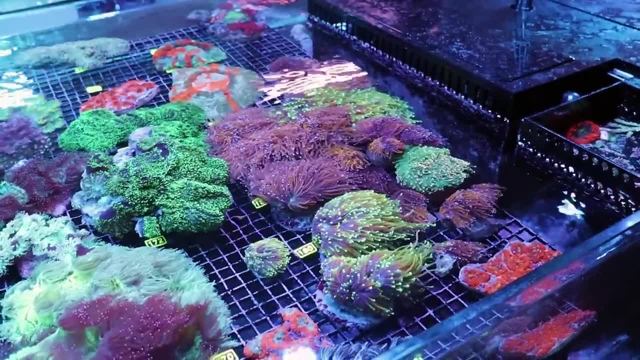 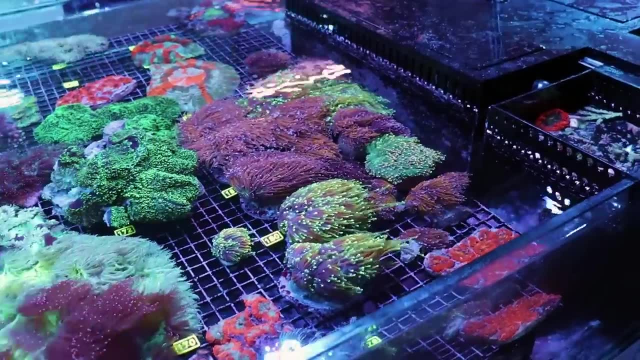 importing so much right now. in the winter months, it's our busy time of the year and it's hard to remember. we bring in thousands of coral, so it's hard to remember which are which, but these ones really, really stand out. we are going to get to frag in shortly. why do we frag them? because they are very 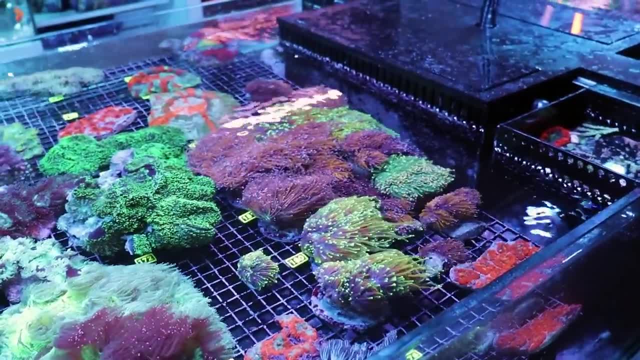 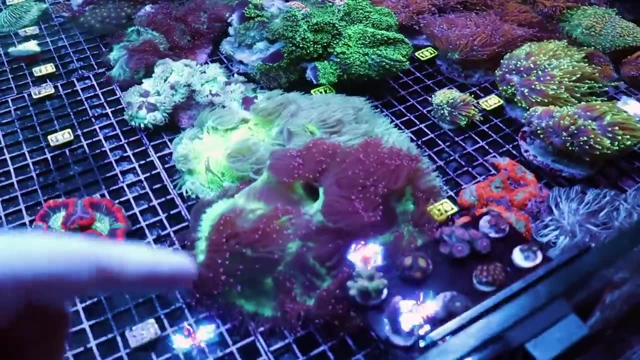 expensive between the cost of the coral. so sometimes you'll hear me say in the video: oh my god, the coral is so cheap and the cost of shipping is what makes it expensive. that is true for some corals, like elegance. you know, if you were to look at a wholesale list of coral, let's say elegance corals from 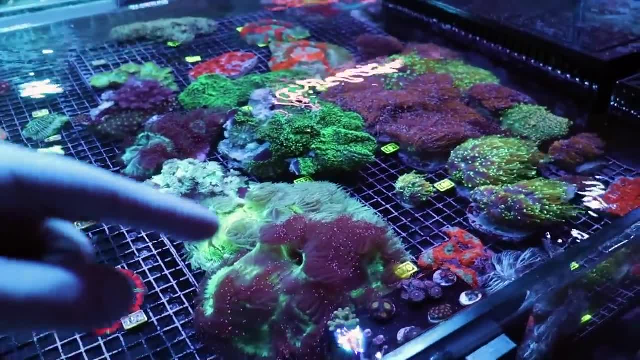 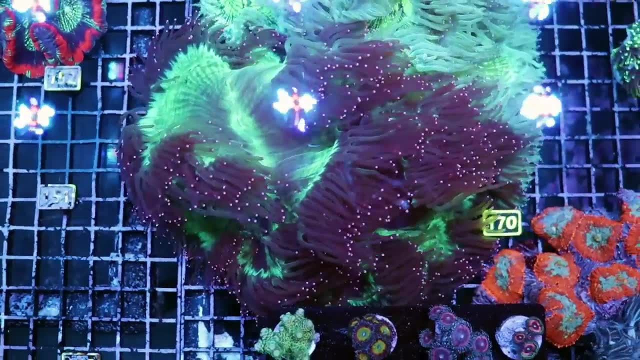 Vietnam. somebody always shouts out the prices there. because you live there, you how much. you please shout out one more time in the comments: how much does an elegance coral like this cost in US dollars in Vietnam? here in Canada it runs about 200- 250 bucks. in Vietnam they're in the backyard. you go out to the 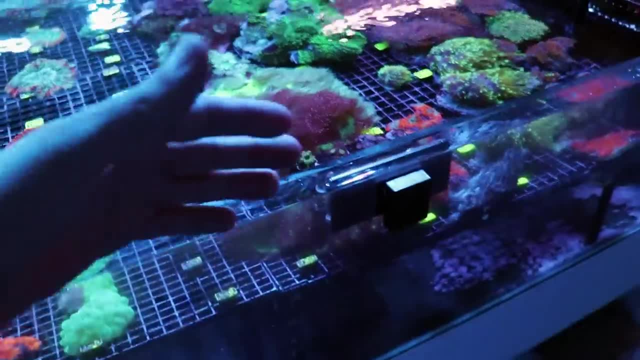 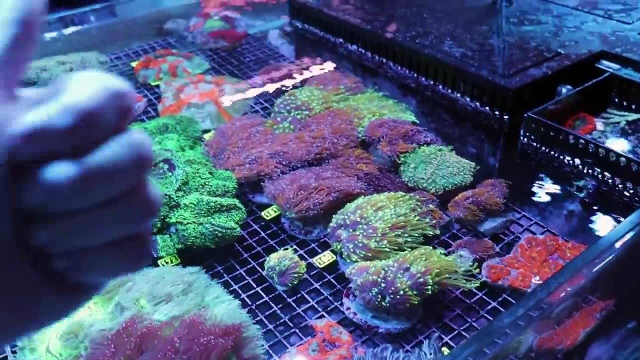 ocean you go and grab one. they're like five, ten dollars us to get them here. the shipping is very expensive. these corals, these torch corals, are not only expensive to ship, they're also very expensive on our wholesale list. they they are not a cheap coral to purchase. they're. not a cheap coral to ship. they do need a lot, a lot of water and there is a I wouldn't some of them die off, so that also gets calculated into the price. the colors are just insane. like I always say, the camera is not gonna pick up. how nice. 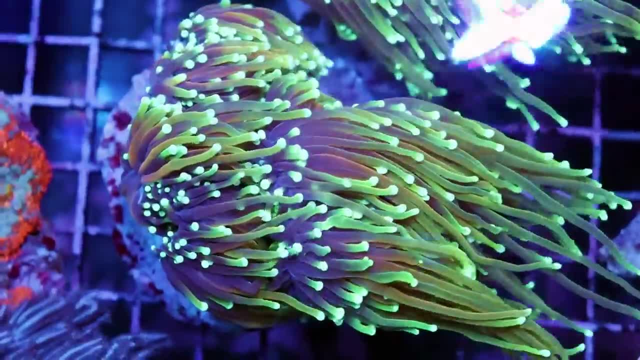 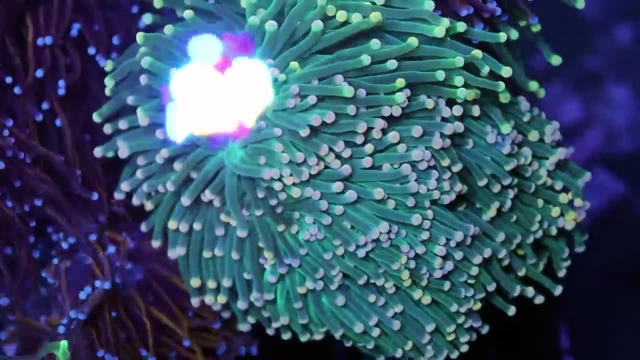 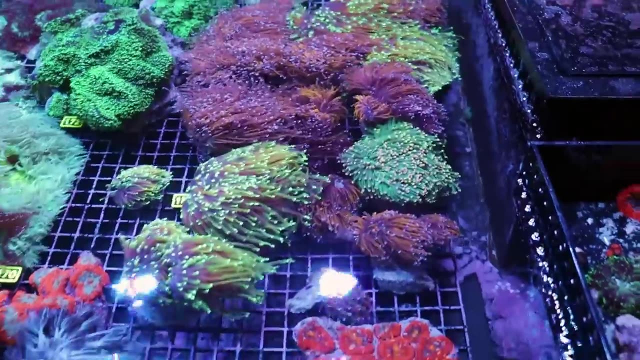 they are and people really want names. they want names for torches. when I started in the hobby, there were no names. this was torch yellow torch. this was orange tip green torch. this was more yellow torch. now we have lots of, lots of names and getting a little bit lost, to be honest. 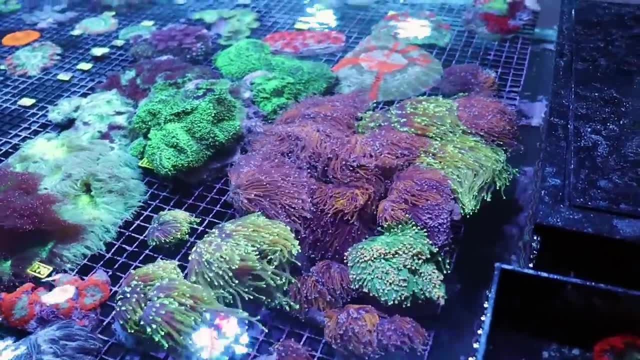 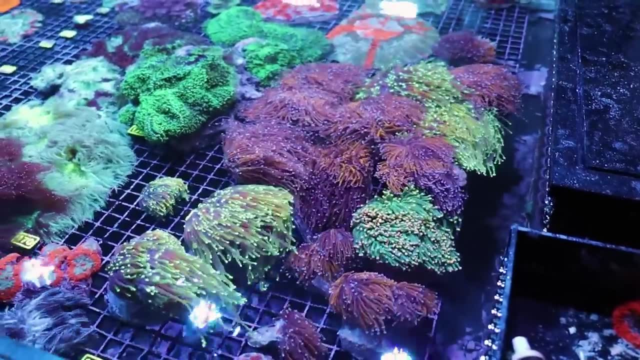 I'm in the industry, I'm in the hobby, I try to keep up with it. people, there's a lot of names for corals in general and I don't know if they serve a purpose for the torch, because when I'm ordering I really only see two on the list. there's 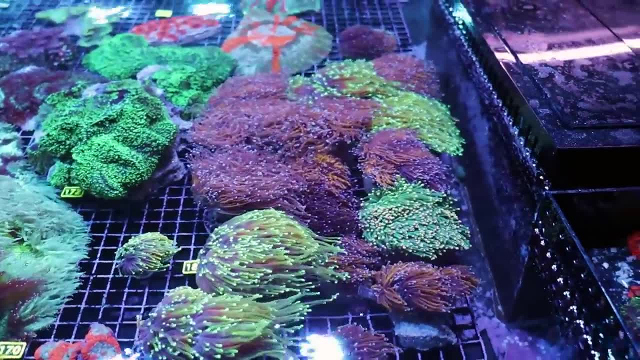 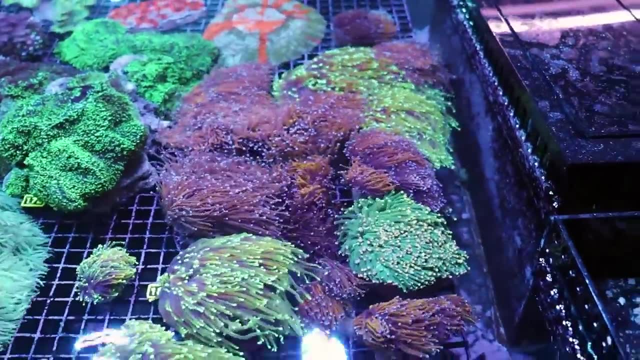 this one and there's this one, and corals can color up and color down. and what I'm afraid, what I'm afraid I'm seeing happen, is this, what I call Indo goal torch. somebody takes it and is able to achieve a better color if you new to the hobby. 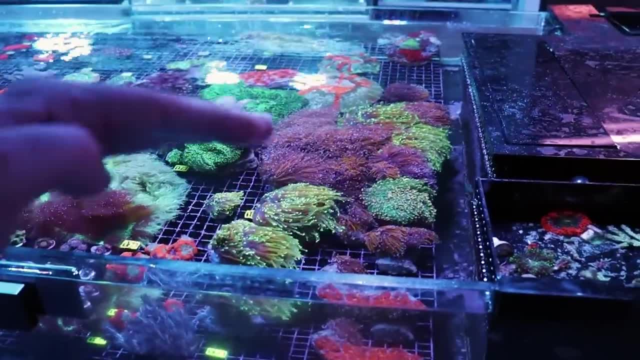 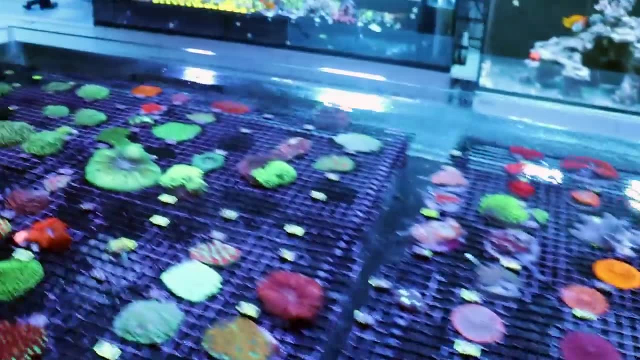 you don't know what I'm talking about. better color, you know. to be honest, I'm not even a true Nordic color. Corals can get better or worse color depending on conditions, especially with Acropora, With SPS corals. maybe I can show you a few here. These ones have excellent, excellent color If 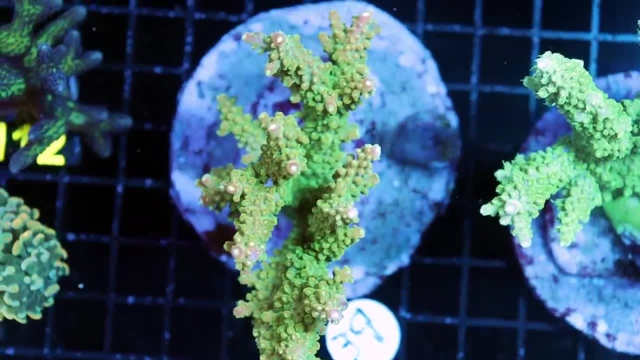 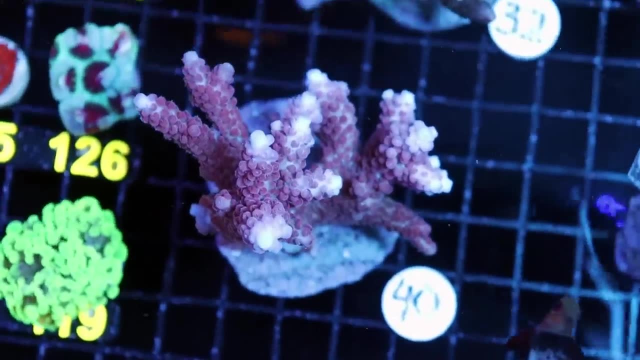 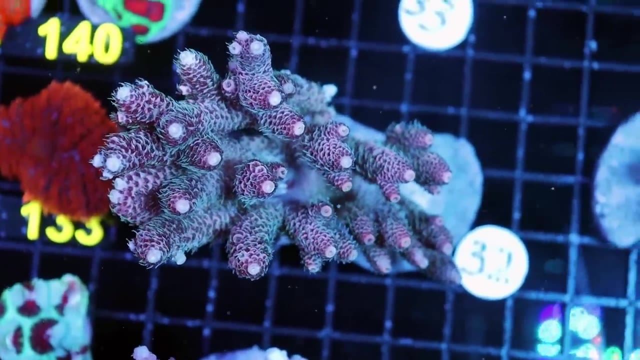 they're not getting the best requirements. no, what am I trying to say? If they're not in the best conditions, they'll brown out. What that means? by browning out, they're going to drop a lot of their. I'm not explaining this properly. They're going to look like crap. 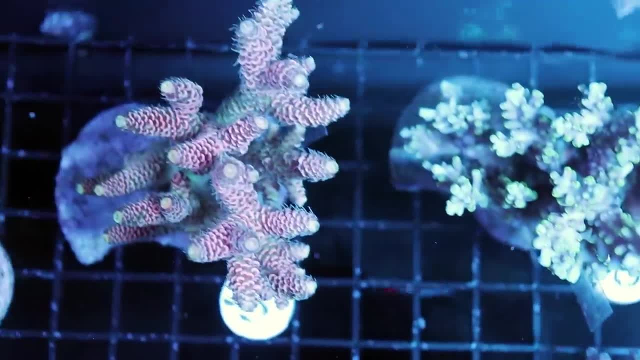 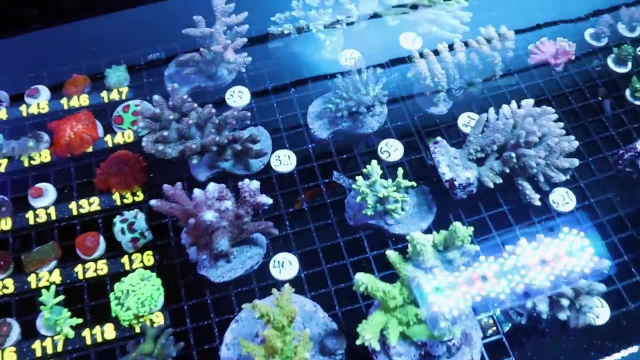 They're not going to look colorful like this, They're just going to go brown- We call them brown Acroporas here in the store- And they're not going to look nice like this one does and like this one does and like this one does. So you can get better or worse color when they're 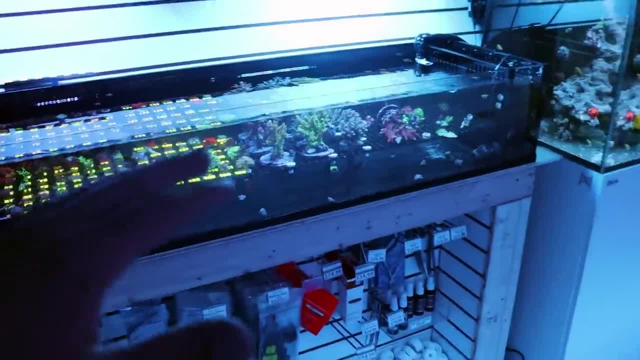 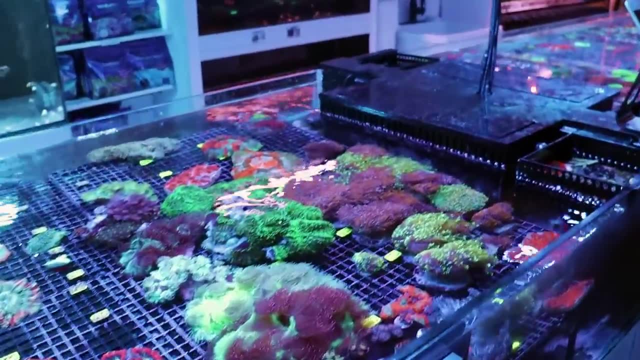 in their optimal condition, the right flow, the right light and the water, chemistry and everything is bang on. The coral is going to reward you with the most insane colors. This also applies to torres Torch corals. Euphyllia can get better or worse color, So what I'm trying to say? this long-winded 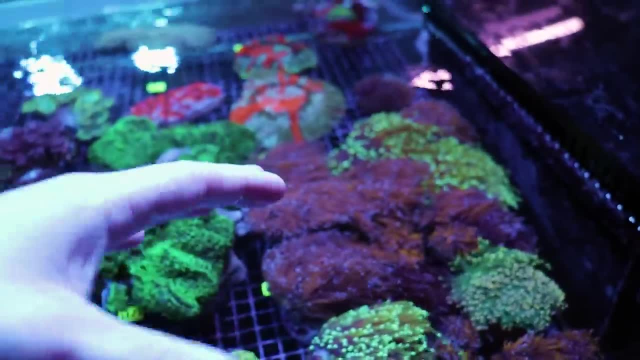 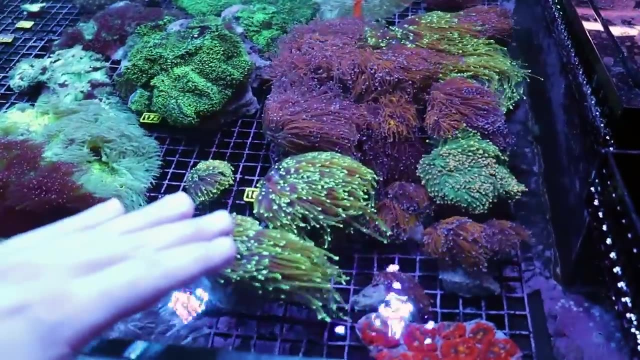 sidetrack is that I think there's just the one: Indo-Gold. Some people get crazy color and then it gets a new name and then a different color in a different tank and another name. I can't keep up. I'm calling these Gold. I'm calling these Dragon Soul. We get a lot of phone calls, Do you? 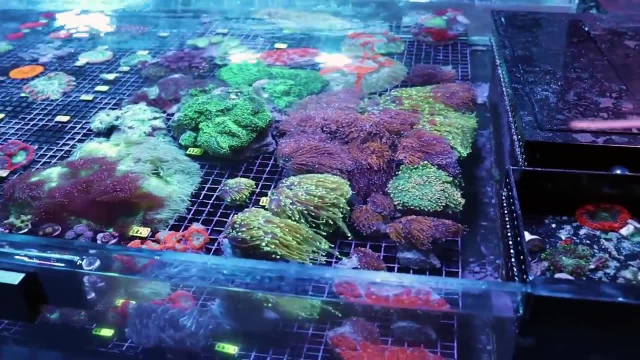 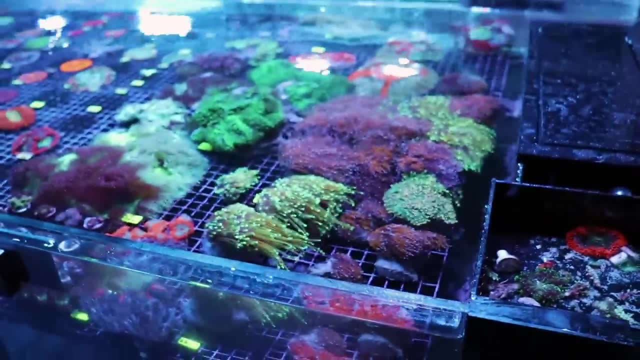 have the New York Knicks? Do you have the Holy Grail? Do you have the Ultra Rainbow Torch? I don't know, These are too many words for an old guy with ADHD. We're going Gold Torch, Dragon Soul. As you know from some of the other videos, I'm trying to move. 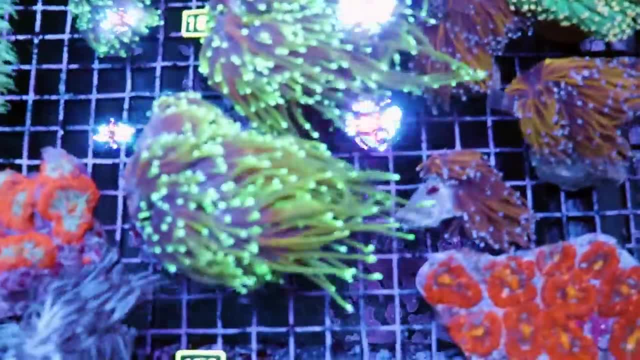 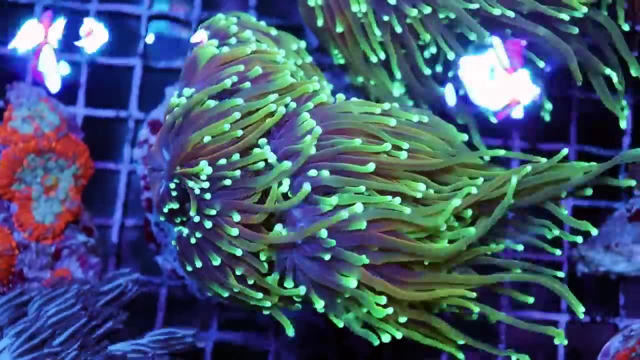 more towards the Latin names of corals in general, So I would really like to just call it Euphyllia Glabarentis. That's the Latin name. I saw the comment Graham Jeffries made in the other video about IDing Acropora and that was a really good point. When we lose the Latin names, when 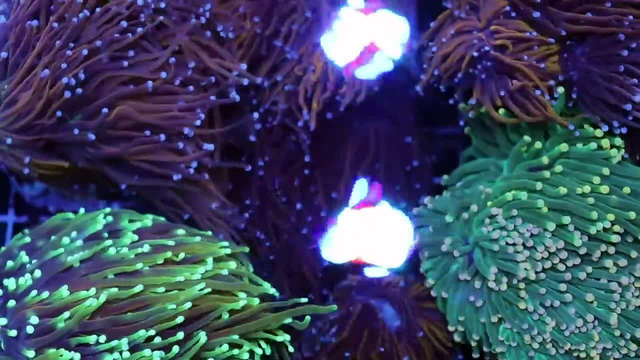 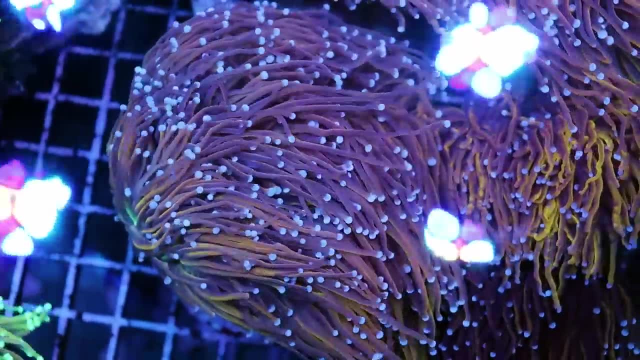 everything becomes just hobby names. it's better, in a way, to have the Latin names, because you can get better care requirements. You can learn- sorry, rather you can learn more about the care requirements of the coral by knowing the Latin name, Because if you go to the corals website, 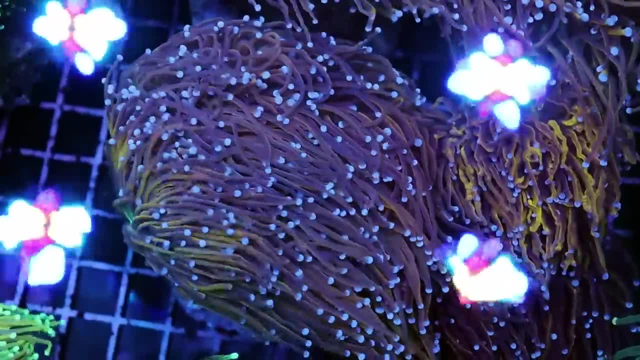 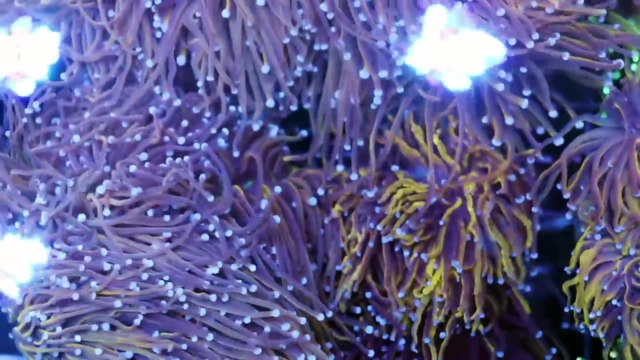 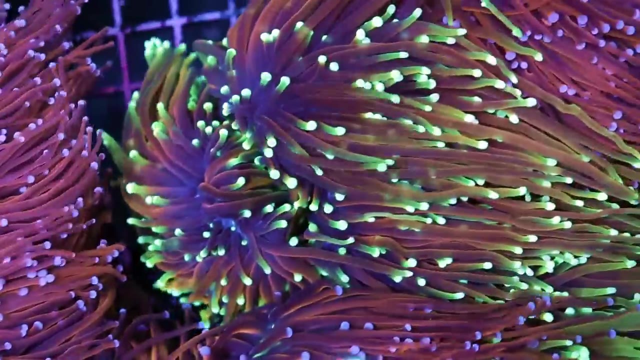 you go online and you type in Hunky Dory Ultra Rainbow Torch. you're not going to find a lot of information on that And it's just sort of a marketing tool Someone's used and attached to a coral to get a higher price. So if you like a coral, buy it. for how it looks. These ones obviously are. 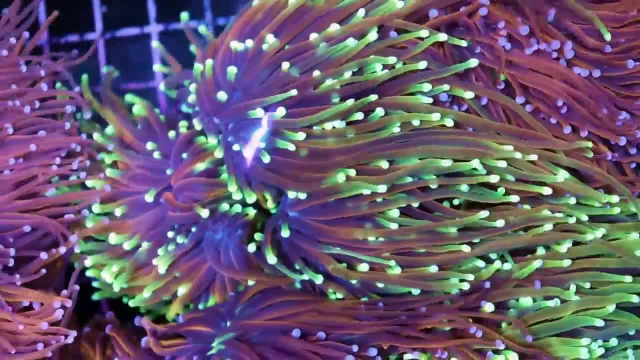 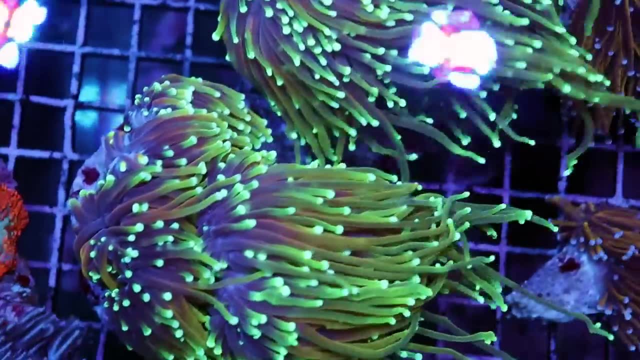 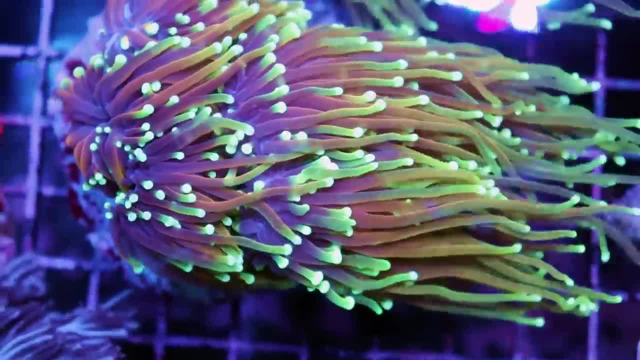 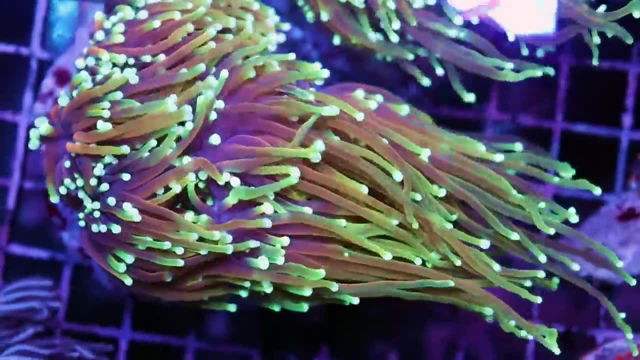 comment that I kind of wanted to make. This one is just outstanding in terms of flow, because this is a question. we get a lot And I'm going to link in the description. We've done two other videos on torch corals that have done really well here on YouTube. The first one is- I think we called it- 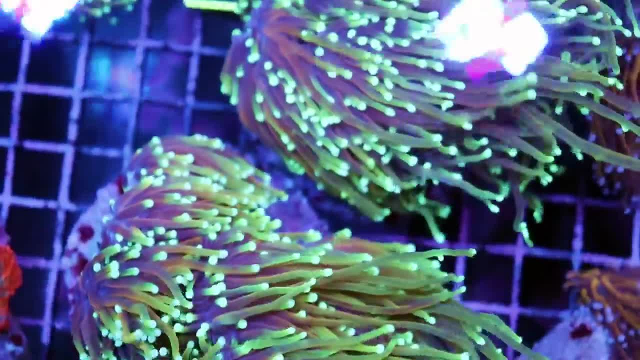 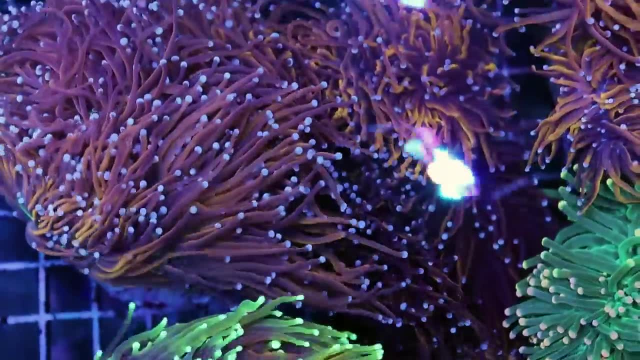 The Secret to Keeping Torch Coral, which is our in the top three of the best or highest performing YouTube videos we've done ever. out of all the- I don't know how many videos we have now up until today- but that one is really popular And I think that's because 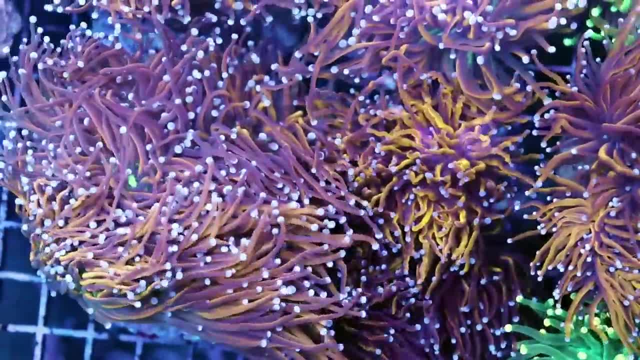 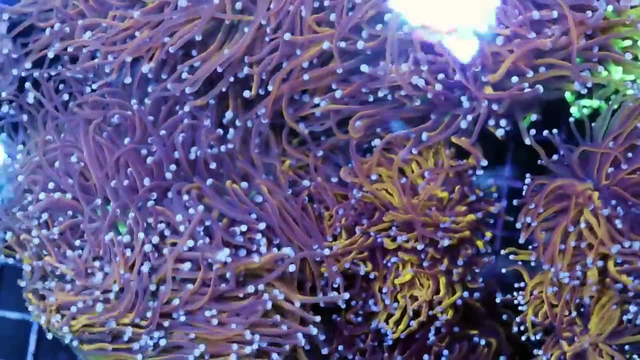 torch corals are really popular and people want to know how to care about, care for them, because they're not cheap. Torch corals, Euphyllia glabarensis, no matter what you want to call them, have gotten very expensive in the hobby. They do fetch a premium price tag, and it's understandable. 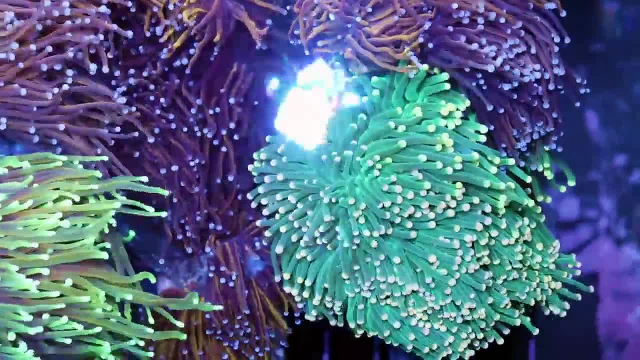 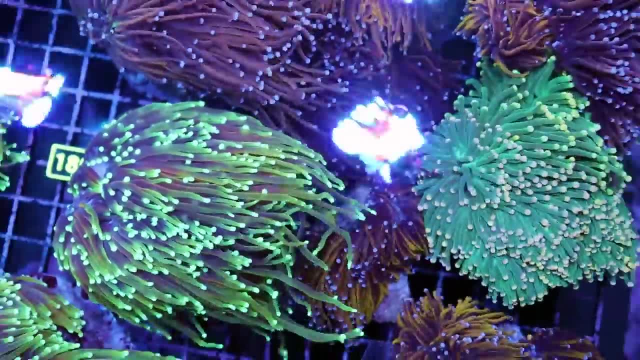 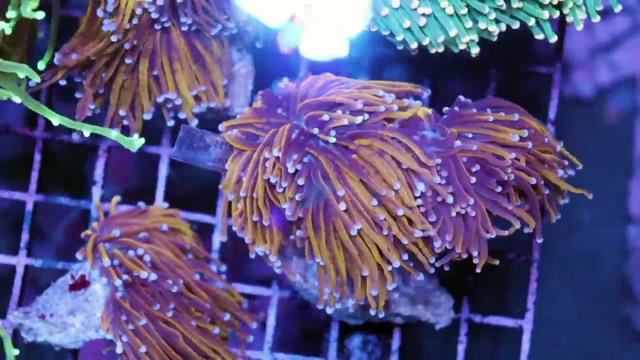 They're beautiful, beautiful corals- And maybe being expensive- I'm just going to throw this out there. Maybe being expensive is kind of good in one way, because it's going to- um, how am I trying to say this? It's going to maybe force some hobbyists to care a little bit more. So we had someone apply to work. 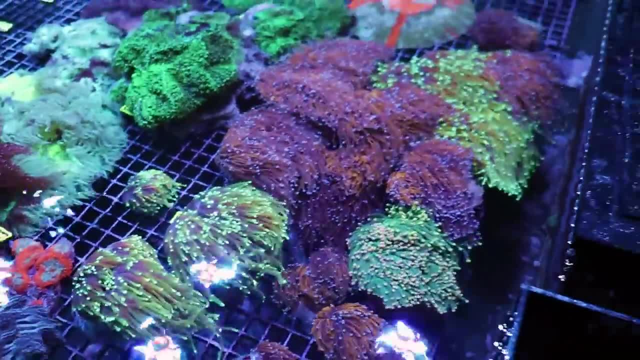 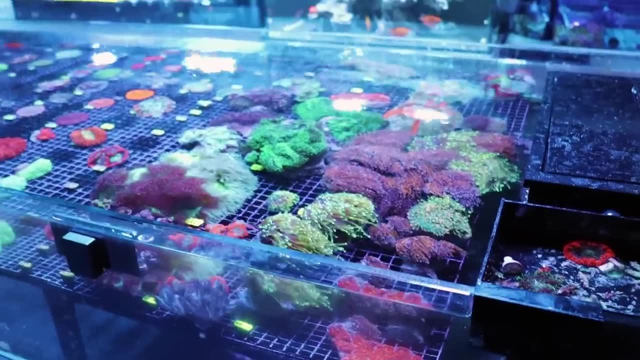 here from Vietnam, very knowledgeable guy. He's actually working at my friend's wholesale operation and I wish we would have got him. He would have been a perfect cultural fit for our team. The only reason we didn't hire him was the timing. He was a student and it didn't line up. So I'm going to 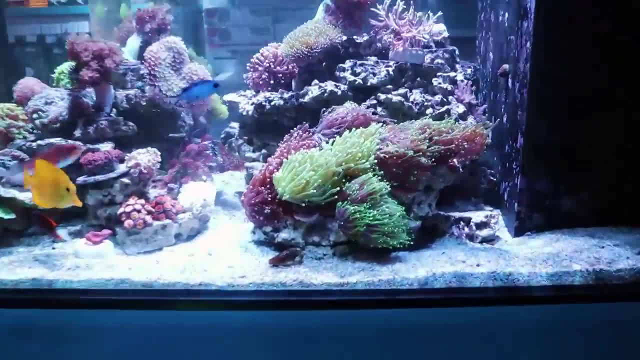 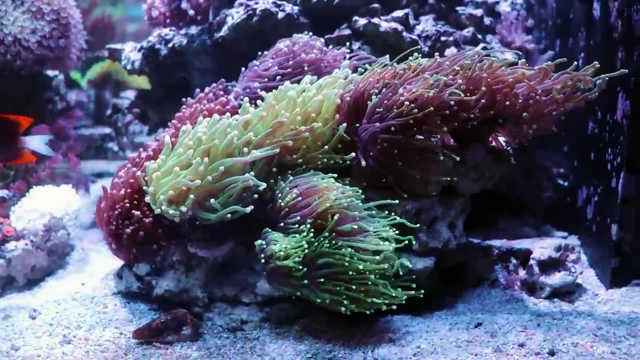 just focus in on these torch corals while I give you my stupid side story. But I wanted him to work here. It didn't line up just because of timing. He was back in school. He was back in school, He was back in school. Hello, Mr Yellow, He was from Vietnam and we got into like a great two hour. 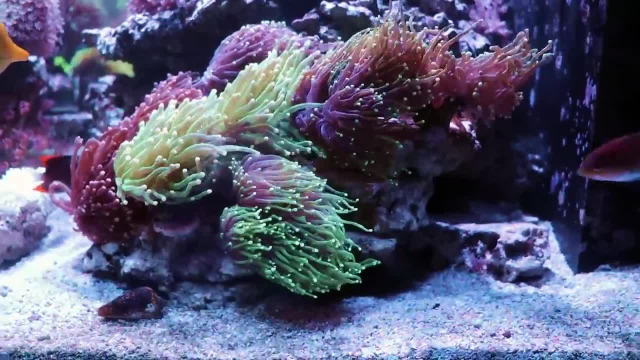 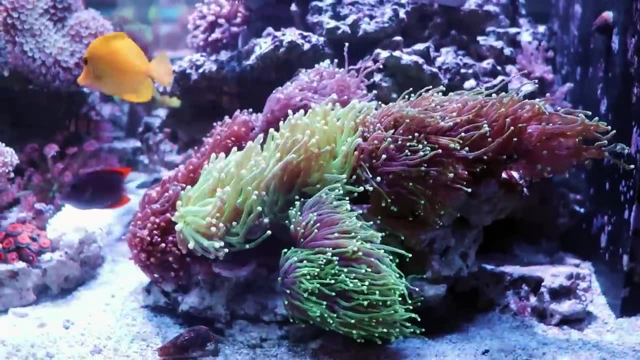 interview here in the store and he was telling us how the hobby works over there. People put in acros, people put carnations, which I never put. They're very hard to care for. They throw in a lot of coral into the tank in a very short period of time because they're so inexpensive. They're 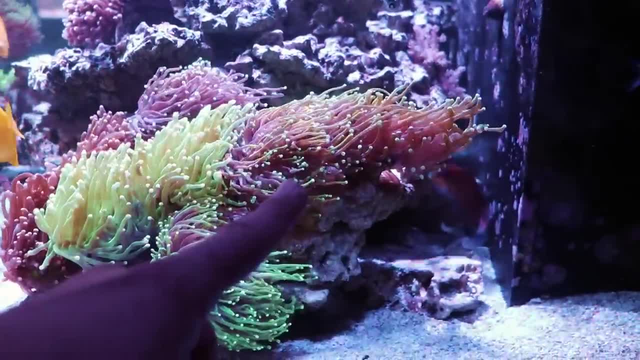 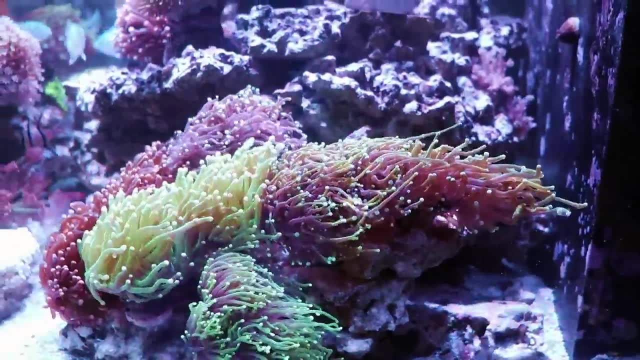 almost like flowers. Think about it. If this is $5,, $5, it's not Here in Canada ahead of this year it's $5.50 for a dragon soul. I think that's about market going rate for ahead of that In the. 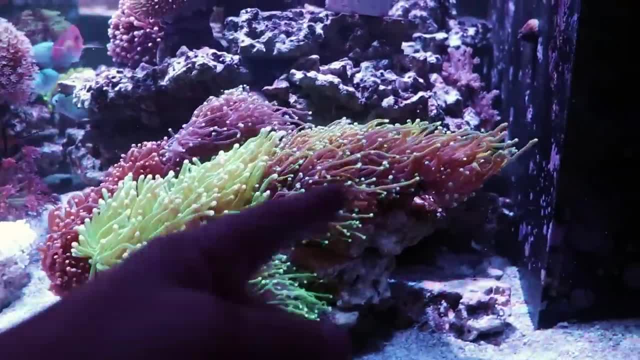 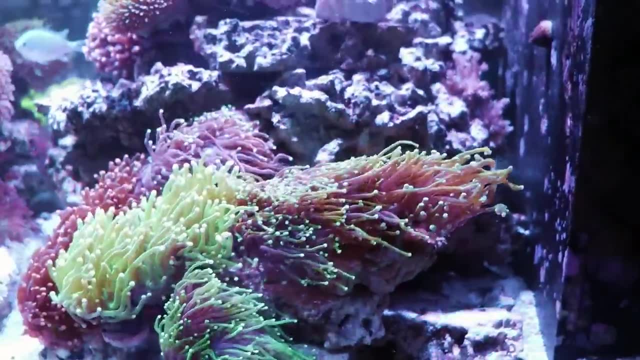 States. I think it's a lot more. Some of the prices are crazy. Now imagine it's $5.. Are you going to care as much for a coral that costs you $5 or $250? The right answer should be: you know. 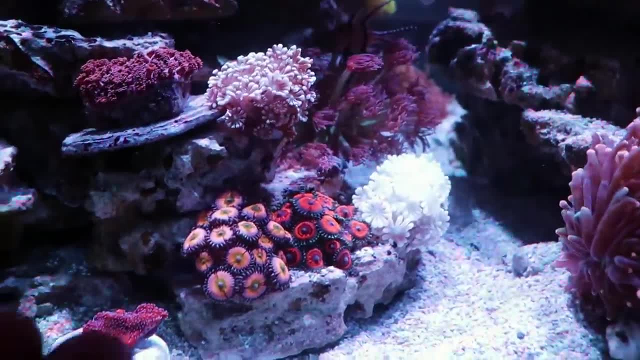 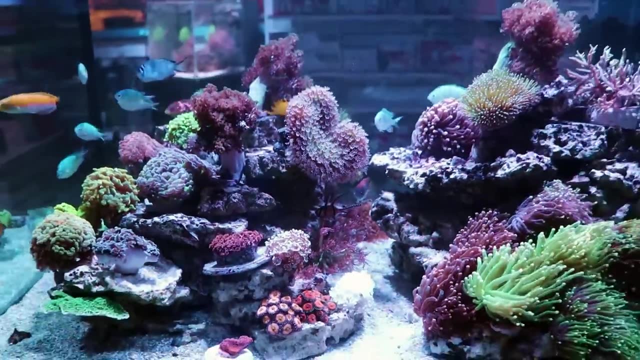 coral is coral, It's alive. It doesn't matter. You know it should be cared for the same way If you spend $500 or $5. I know that when I've put my first Walt Disney frag in a tank years ago. 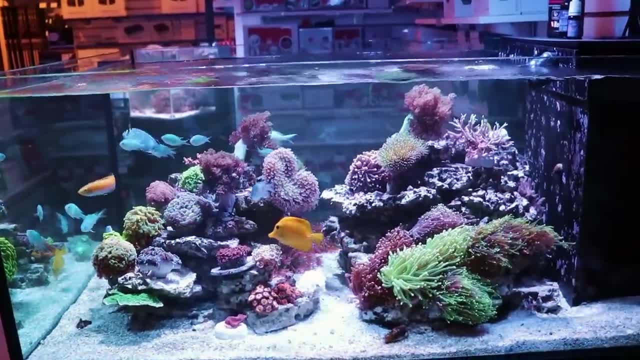 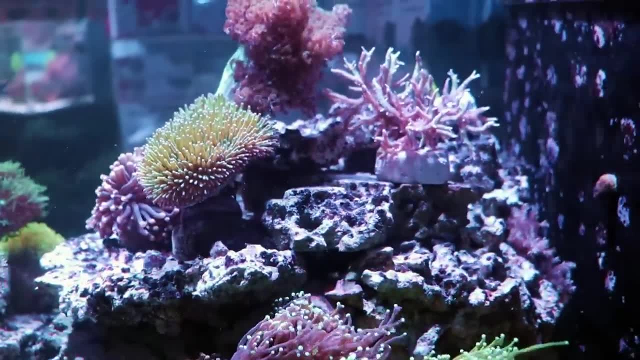 I'd wake up in the morning and the first thing I would do- I mean my feet would touch the ground and I would run to the tank and go check on the Walt Disney, because I put $500 in that piece and I was, you know, very nervous about it. I don't know if anyone else has that sort of experience where 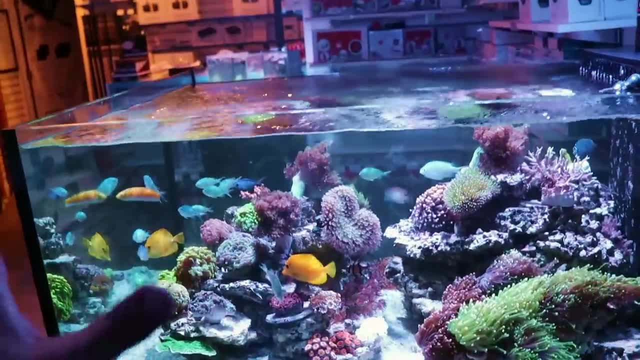 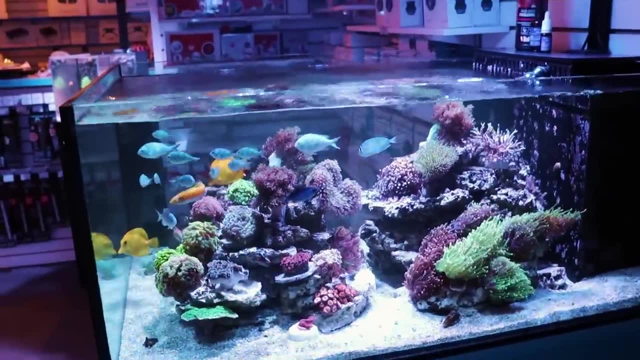 you have a very expensive coral and your eye is just drawn to it and you design and plan the whole tank around your home wrecker or your dragon soul. Share with that in the comments below. if you know what I'm talking about, Maybe maybe you understand. Maybe you don't, I don't know if you're in the 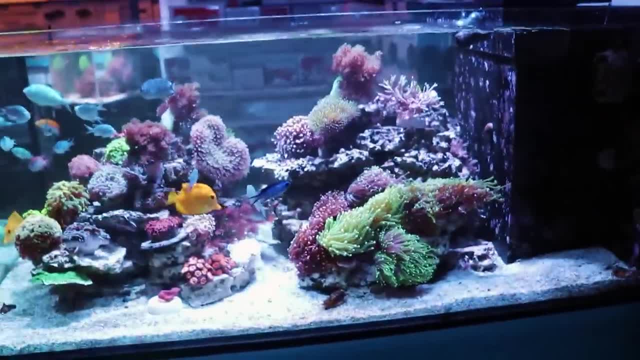 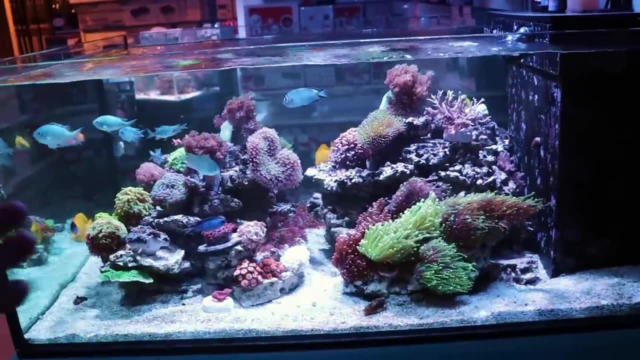 same boat. I feel like there's a tendency to you know if you're going to spend more money on it, you're going to pay more attention to it, You're going to care about it more. This guy was telling me that in Vietnam $5, you know, let's say elegance corals five, 10 bucks. It was almost. 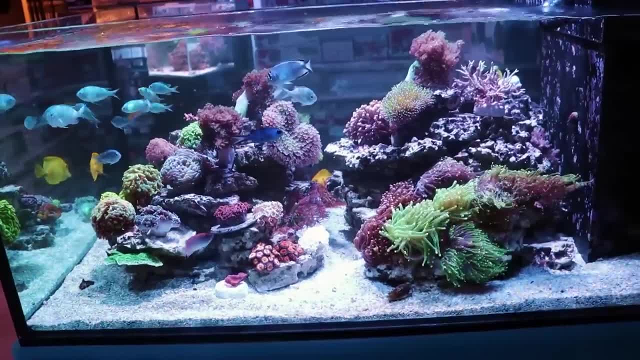 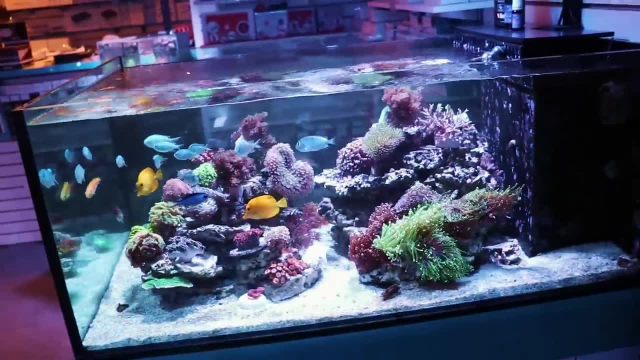 like fresh cut flowers. You would add them If they died five, six months later. it's so freaking cheap. You go out to the store and with 20 bucks you got four new colonies. Look at that. Your tank is back to normal And um, that's what I'm trying to say. Maybe the fact that they've gone more. 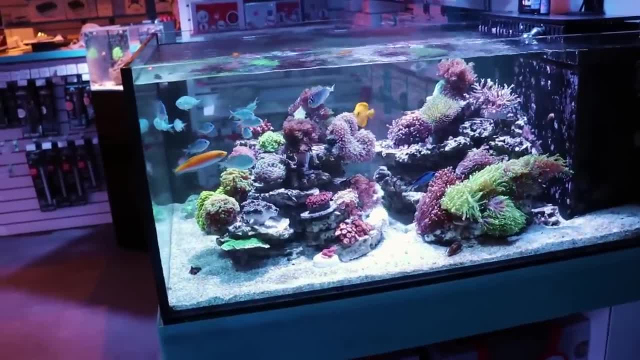 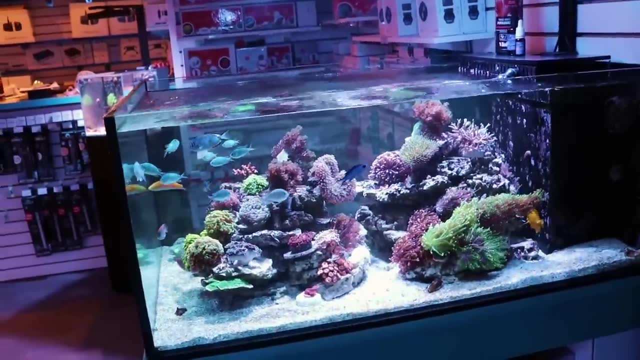 expensive. maybe it's good in a sense not good for your wallet. Obviously, you're spending more money. Maybe it's better for for the corals. Maybe it's better for the hobby that you're going to pay more attention because it's not cheap- $250.. That is not a cheap coral. that. 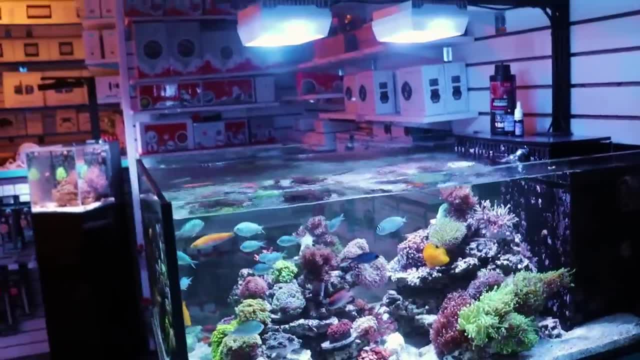 if it's cheap for you, kudos, I'm, you're in a great industry, I'm- let's, let's team up and we'll do something else. for most people That's not cheap. That's quite a bit of pocket change. And I think I'm just trying to share. It might be good in one regard: When I first started torch, I used to buy them wholesale for $10 a head and I'd sell them $20 a head all day long And I was on cloud nine. That was amazing. Uh, those days are so, so, so far gone, Very, very far gone. 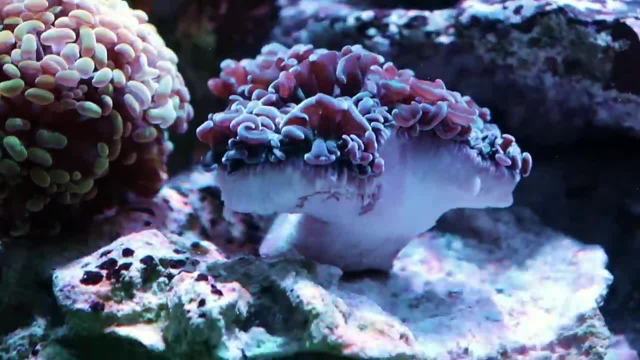 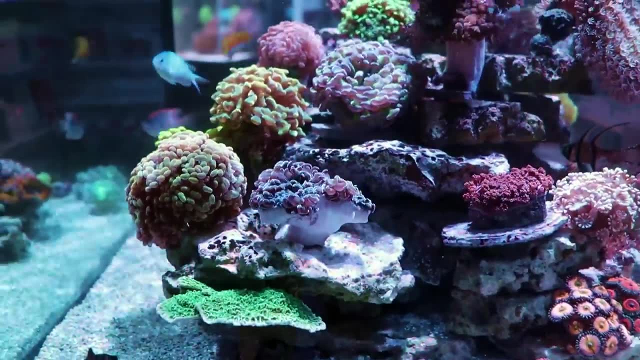 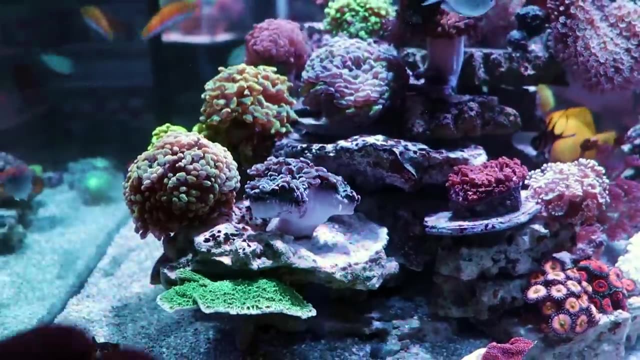 Why are you not opening yet, mister? Hmm, I just added this guy recently. This is a blue- yes, blue- hammer coral. It was here available for purchase in the store for 125 bucks. Nobody wanted it, And then we put it on sale for a hundred bucks. Nobody wanted it, So I decided. 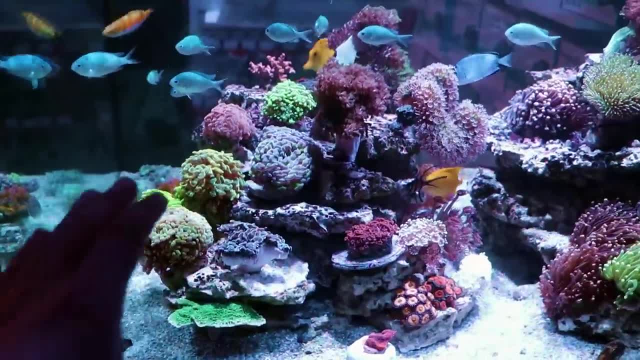 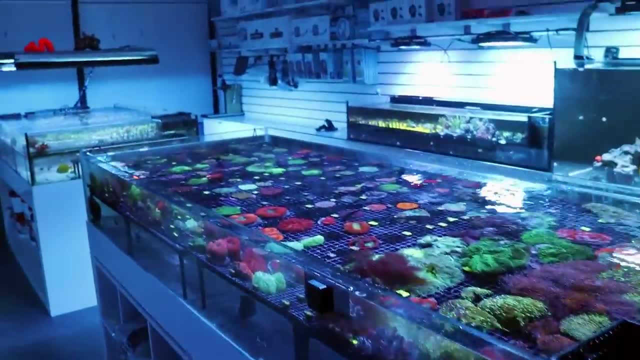 to keep it. Sometimes people's eyes, I think, just gloss over stuff for sale. The hamburger garden is coming along really nicely, but I think people are drawn to the really really bright stuff And sometimes the subtle and weird things that are really nice sort of in between. why is? 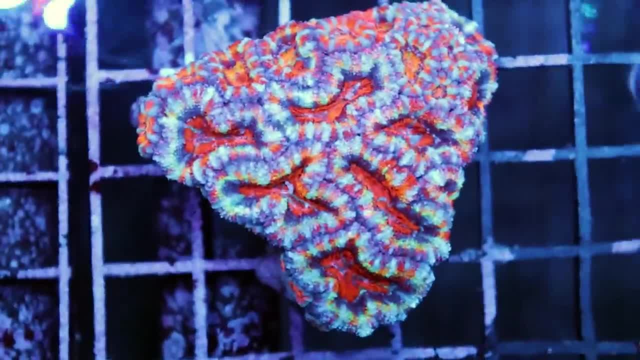 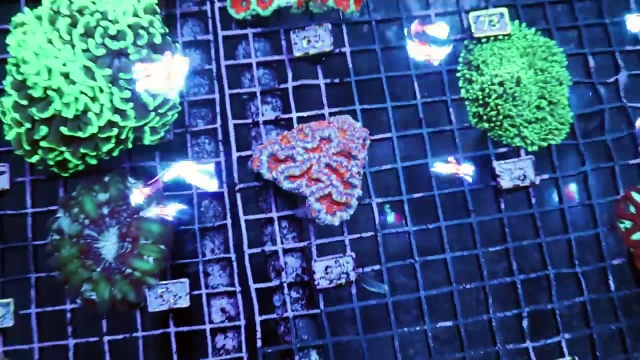 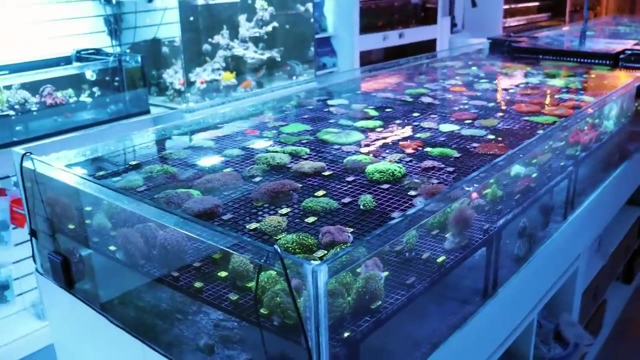 this still here? Look at this. Why is this still here? I think it's a hundred and change on the site. This a can is crazy. This thing is nuts. but sometimes there's too much going on or maybe the staff is distracting and we're doing videos in the store and you miss it. So I'm kind of glad. 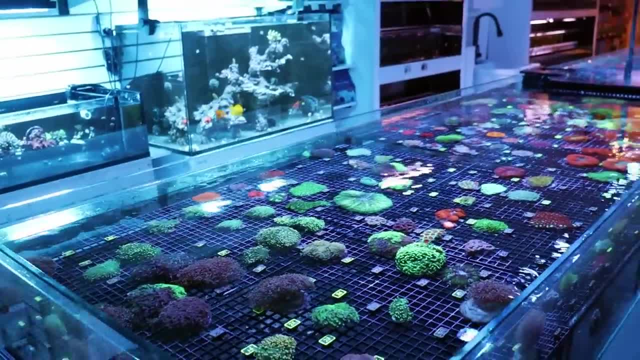 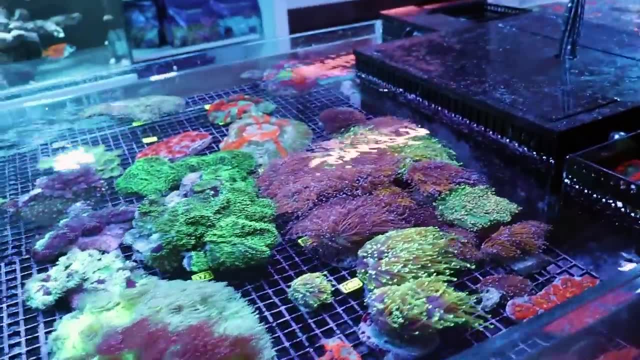 it was sitting right there. I think it was like number 37, 35.. I'm kind of glad that nobody saw it and I got to keep this beautiful blue hammer. But today's video is not about blue hammers. It's about torches and we are going to frag them up. So if there's any of the ones you like here, 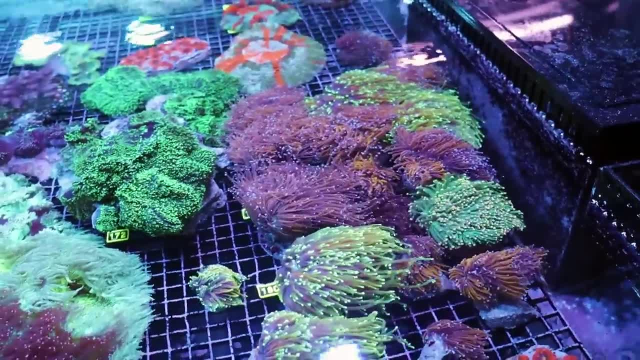 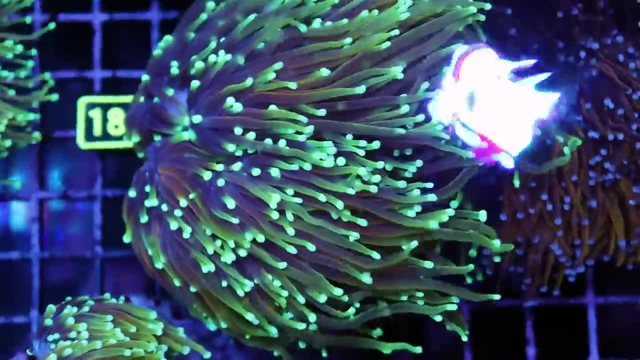 we are gonna- I think Dylan's going- to cut them this week. We do like to give them about, I would say about a week, maybe four to seven days, just to make sure that they're nice and healed And looking good, because we only want to sell healthy corals and make sure that they're going. 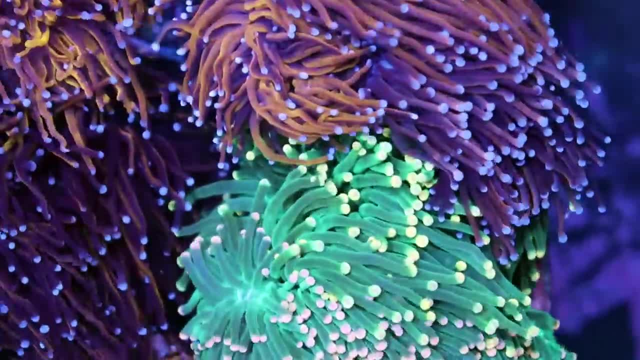 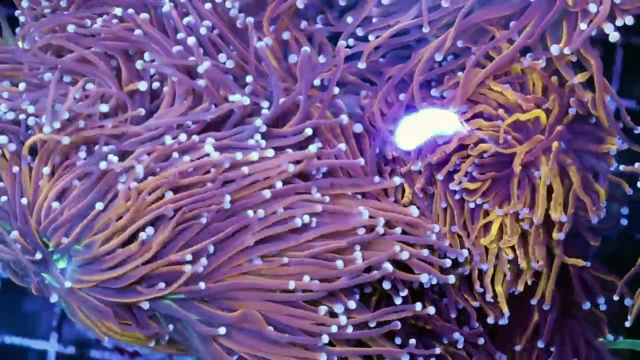 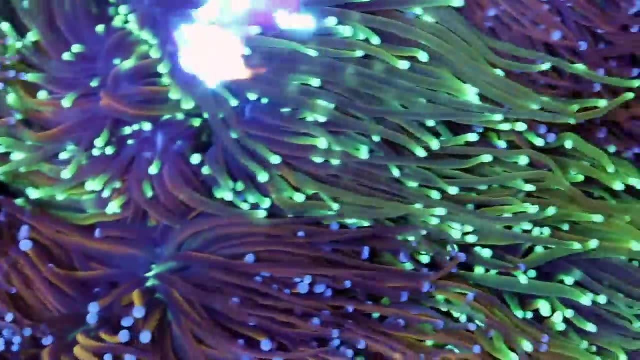 out in their best possible condition. So look for these on the site soon, If this is something you're after. they're not going to last long, That I can tell you for sure. I don't make a lot of promises, but I can promise you these are, these won't last long. So I think we're going. 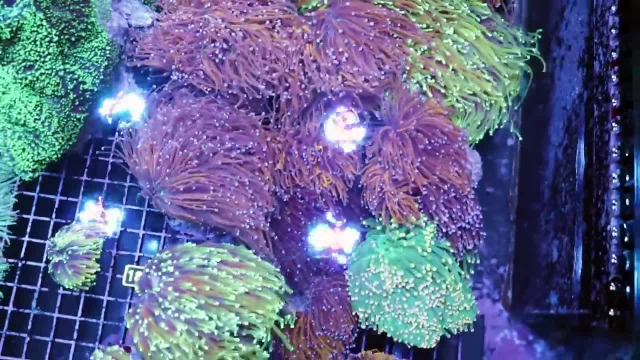 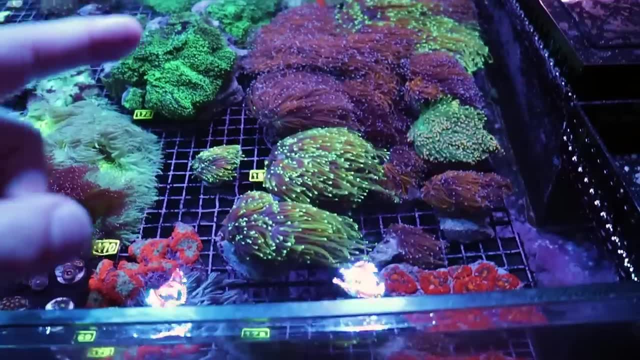 to wrap it up, I think that's about all I can say about torch corals and ranting on coral names and sharing some little sidetracks and experiences. I, like I said, I will link in the description the care requirements for these. It is it might be time for an update on that video. I think we 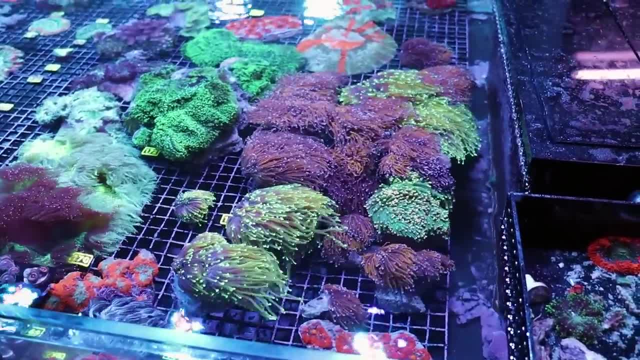 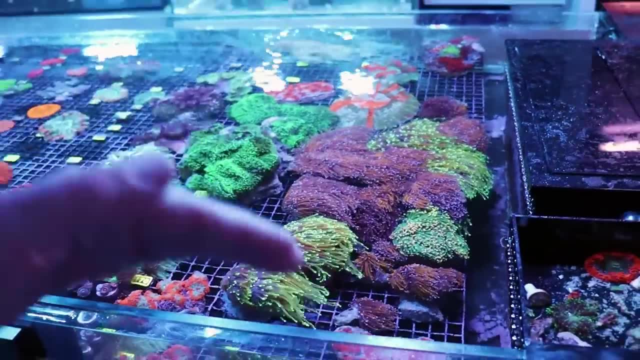 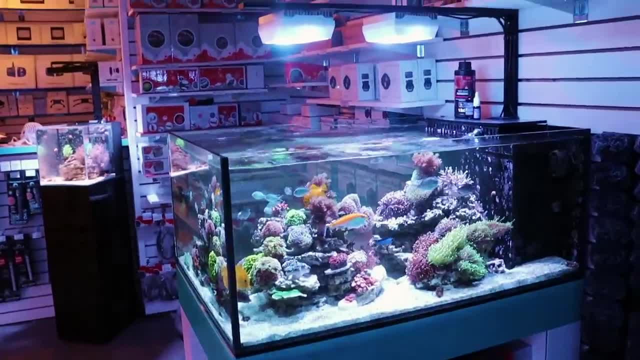 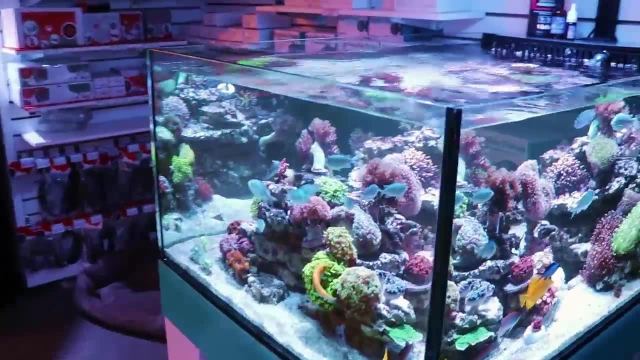 that you may have. I'll be happy to answer any questions that you may have, And unscripted. So there are times when I do miss things, something, sometimes something very, very simple. So I do appreciate those comments below And we do have a giveaway coming up and you don't have to do. 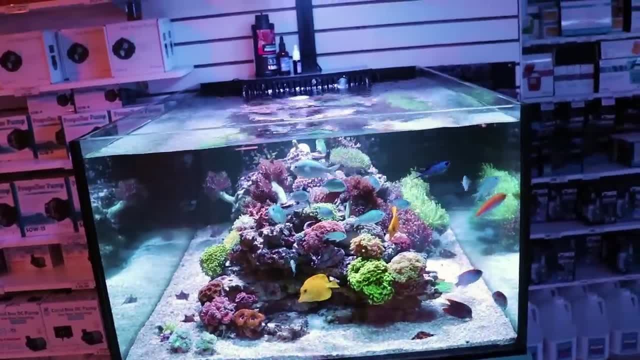 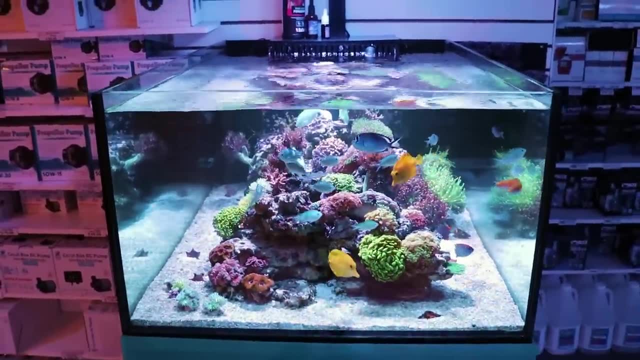 anything actually to win this giveaway. You'll see what it is. It's something I think it's cool. You guys will see. it's based on comments people have made on the past six months And we're just going to simply send you something for free in the mail. It's, you'll see, I'll, we'll talk about. 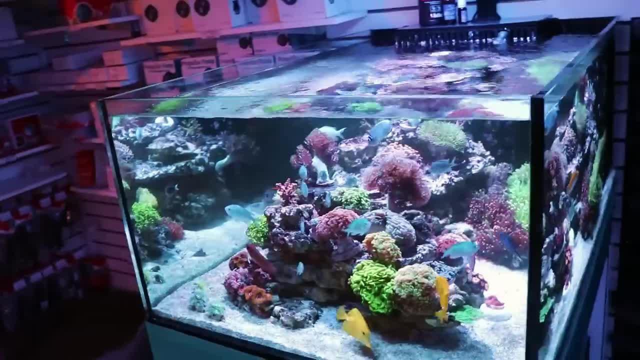 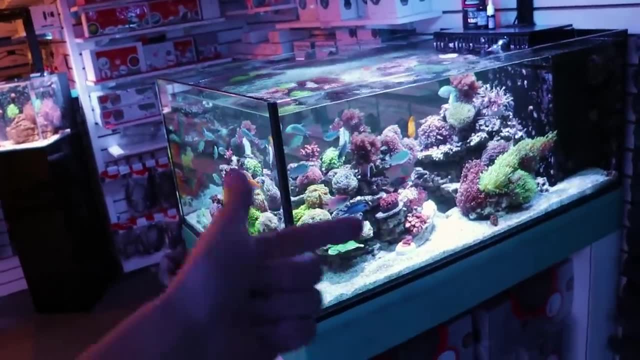 it when they come, And then I'll shoot some, some messages out there and try and get your addresses. I know somebody's in the, somebody's from the Ukraine, Somebody's from Texas, So we are going to ship them around the world, these things. It's you'll see. you'll see, Stay tuned and come back here tomorrow If